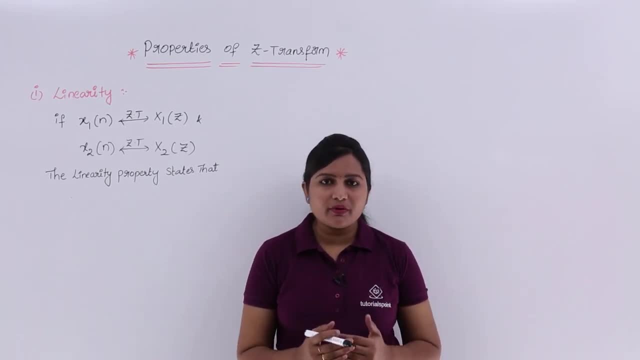 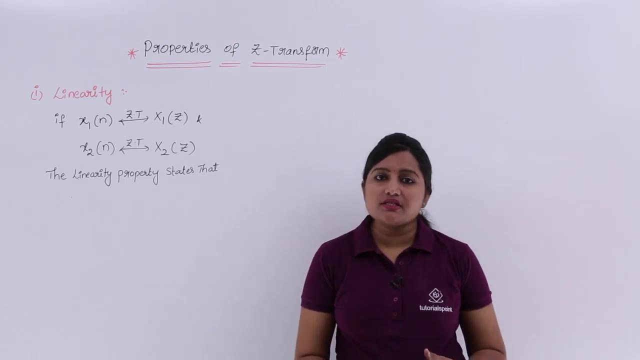 In this video we are going to discuss some important property of Z-transform. that that means linearity property of Z-transform. In next 2-3 classes we are going to discuss that important properties of Z-transform. So in this class especially we are going 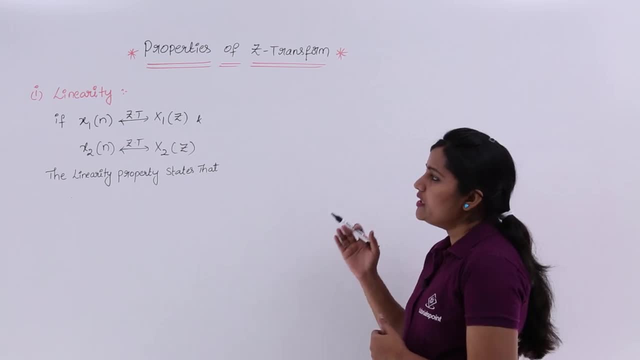 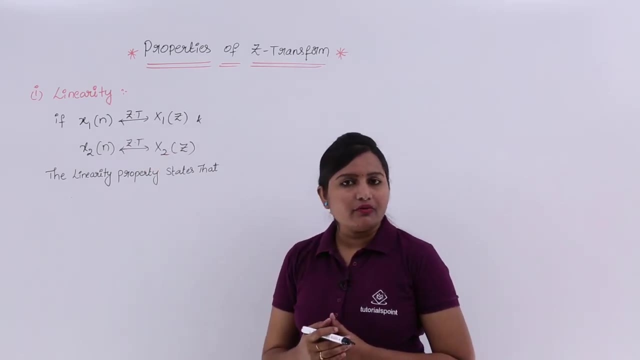 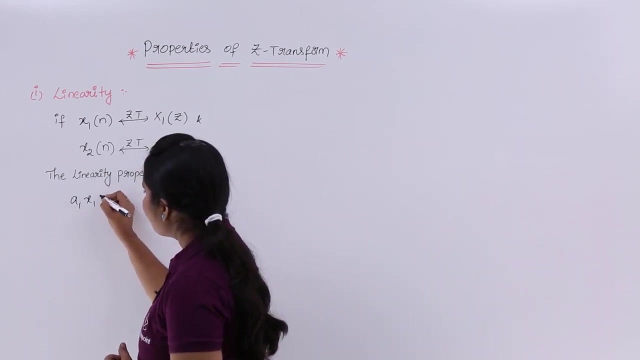 to discuss linearity property of Z-transform. So here what this linearity property states means. So if X1 of n and X2 of n are two discrete time sequences with Z-transforms X1 of z and X2 of z respectively, then linearity property states that A1, X1 of z, A1, X1 of 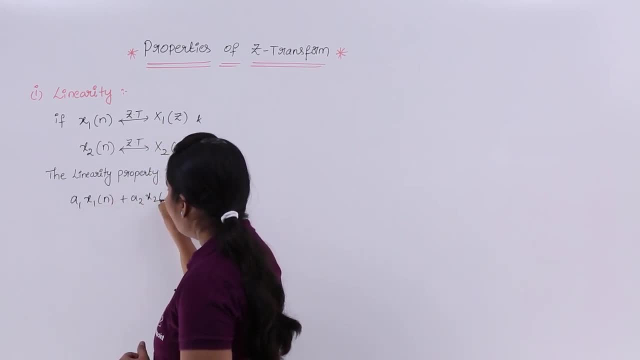 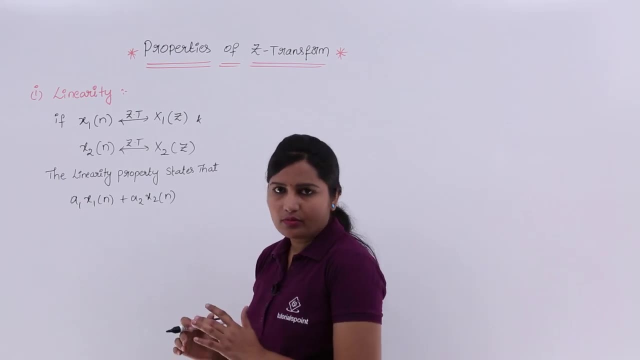 n plus A2, X2 of n. This is a collective, discrete signal. We combine these two signals and transform it. Then the relationship between X1 of n and X2 of n is A1- X1 of n. So this is a collective. 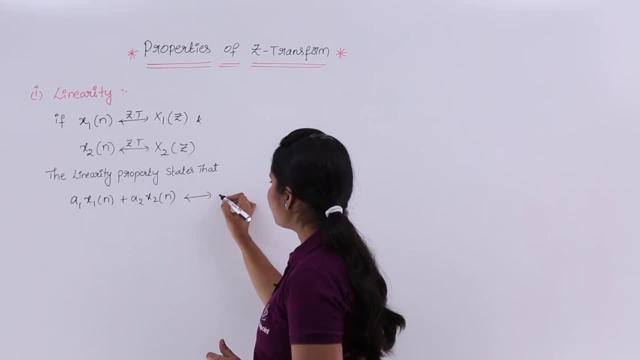 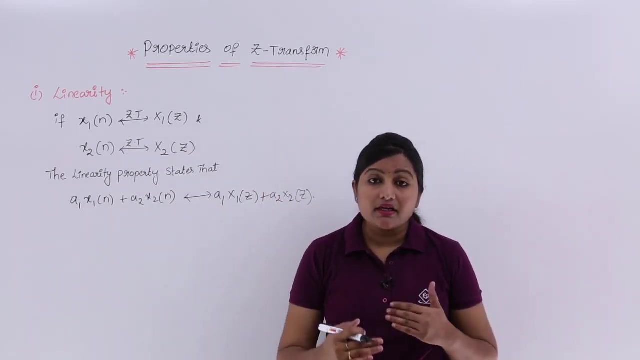 transformation of that combined transform. with this transforms will be A1, X1 of z plus A2, X2 of z. So like this we are going to get the transform. So if you are combining your signals in time domain and you transformed by using z-transform, 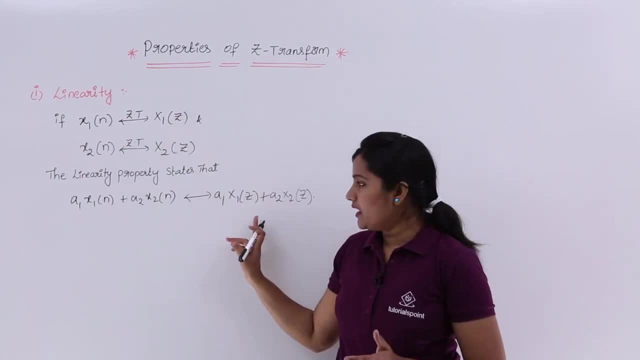 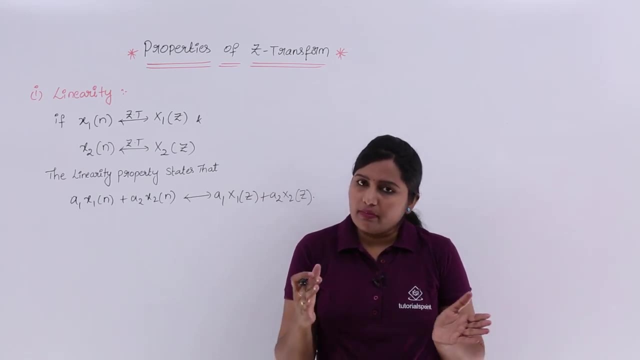 then you are getting the same. like this: A1, X1 of z plus A2, X2 of z. That means individual transform. So if you combine individual transforms, or if you combine signal and in time domain itself and you consider z-transform for that, you are getting the same. So this is the. 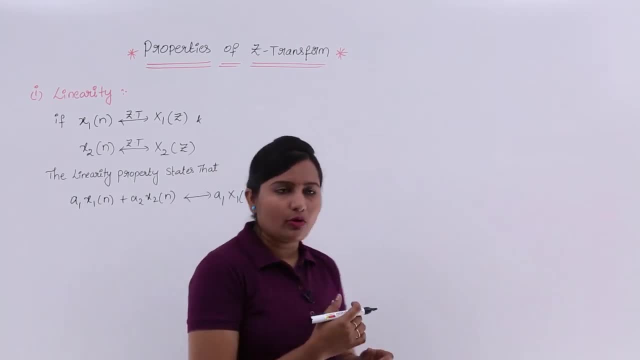 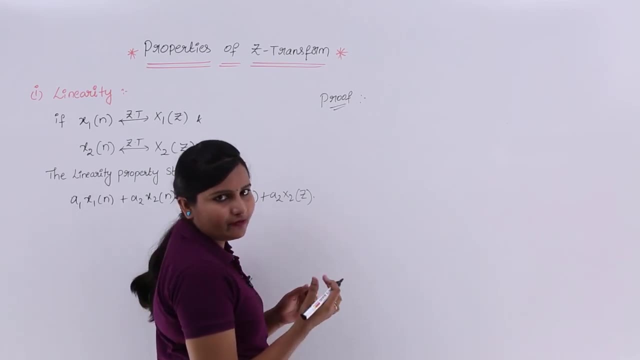 theme of linearity property. Now we are going to prove this property. As a proof, I want to consider general z-transform of any X of n. So here I want to consider z-transform of X of n. Z-transform of X of n. 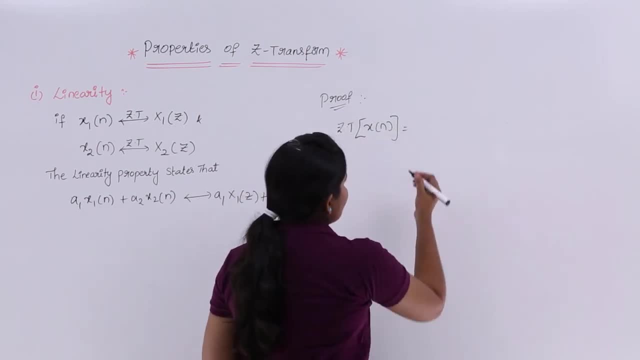 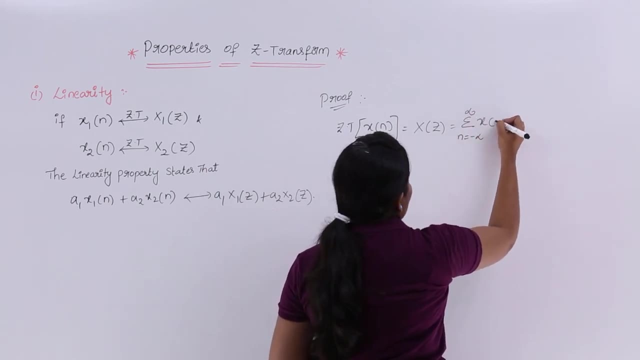 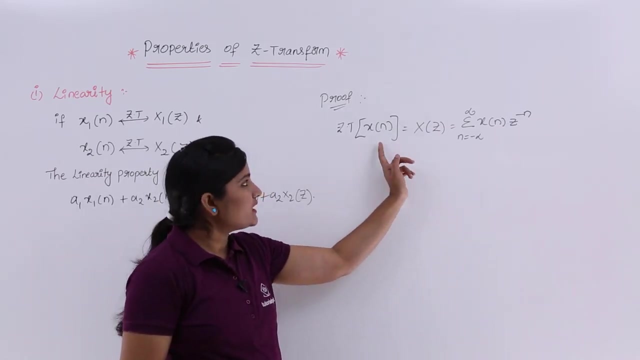 General equation of z-transform of X of n, of Z transform of X of n is equivalent to X of Z is equivalent to summation, n is equivalent to minus infinity to infinity, X of n into Z power minus n. This is the general equation of Z transform. to calculate the Z transform of any discrete sequence: X of n. Now what? 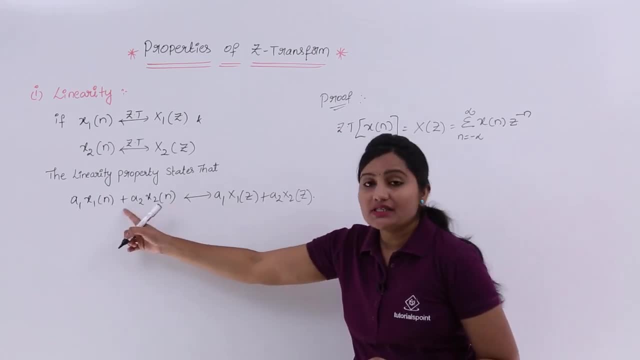 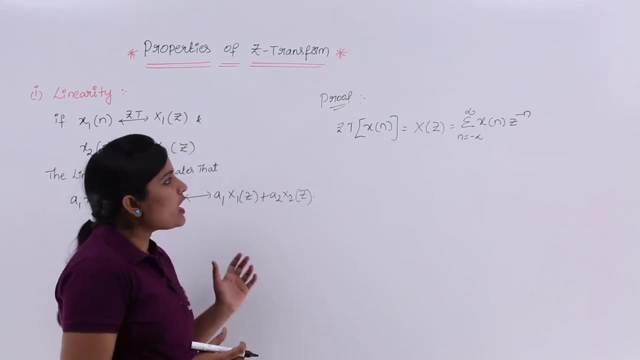 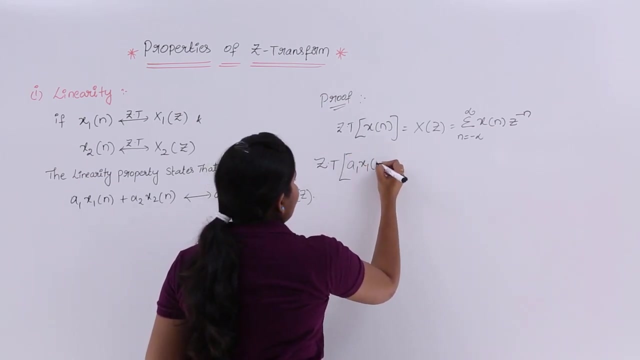 we need to prove. We need to prove the Z transform of this combined sequence is equivalent to this. So, addition of individual transforms we need to prove. So I am considering that combined signal as my signal to get the transform. My signal now is X1 of n plus a2, X2 of n. this 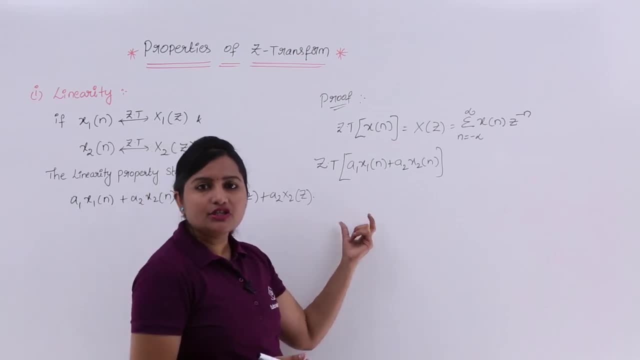 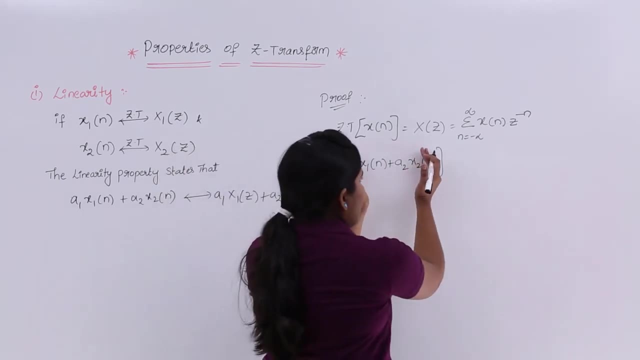 is my signal. So this signal, I need to get Z transform, I need to calculate Z transform for this combined signal. So this signal I am replacing in place of X of n, Why? Because now my signal is 0.. So this is my signal. So this is my signal. So this is my signal. 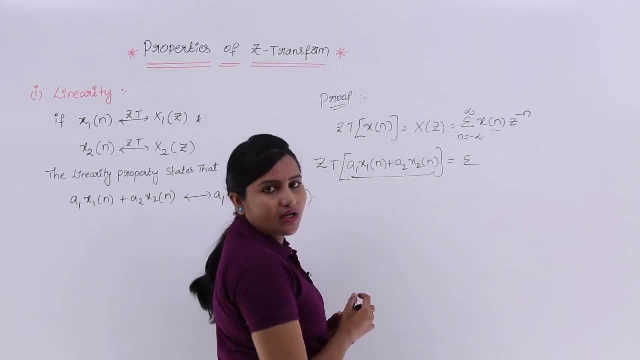 Now my signal is not X of n. My signal is a1, X1 of n plus a2, X2 of n. X1 of n is one signal, X2 of n is another signal. by combining those two signal we will get another signal. 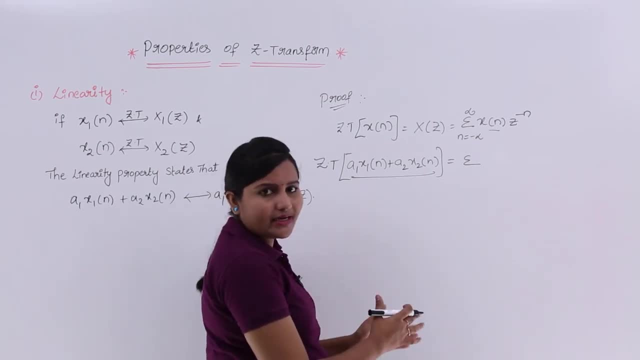 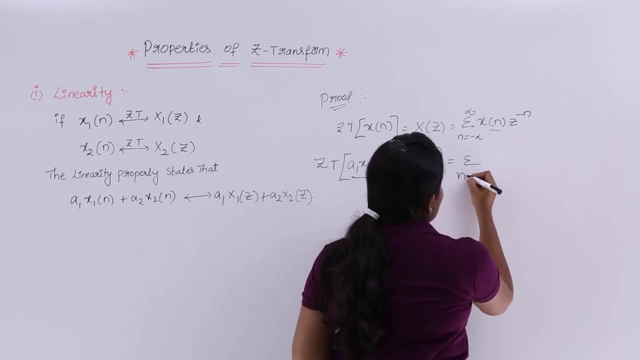 For that special Z signal, that means for that third signal, combined signal. I want to find out my Z transform. So that is why I am replacing in place of X of n. So n is equivalent to minus, infinity to infinity. Where is the first one? 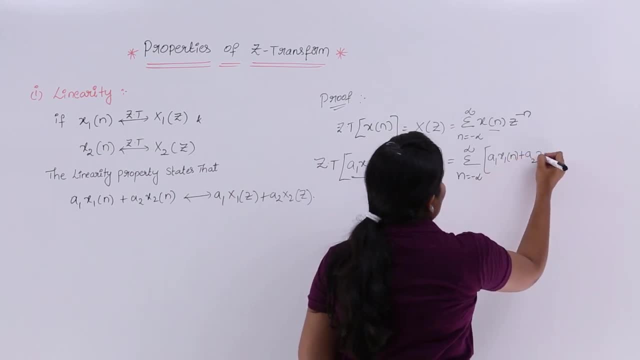 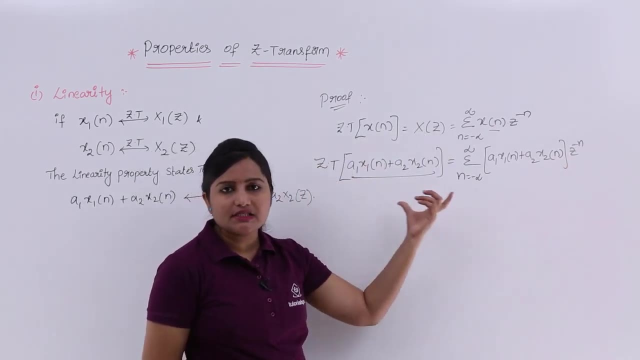 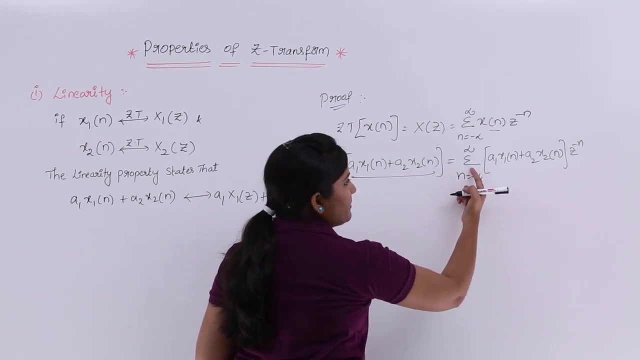 a1, x1 of n plus a2, x2 of n into z power minus n. This will be your modified equation to calculate z transform of this combined signal. So I am separating these two terms into two different summation and into z power minus n terms. So you can see summation: n is equivalent to minus. 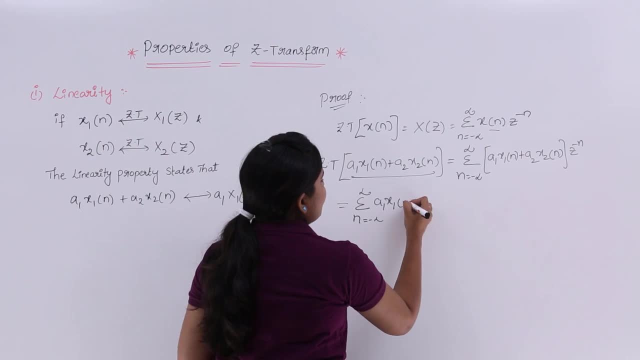 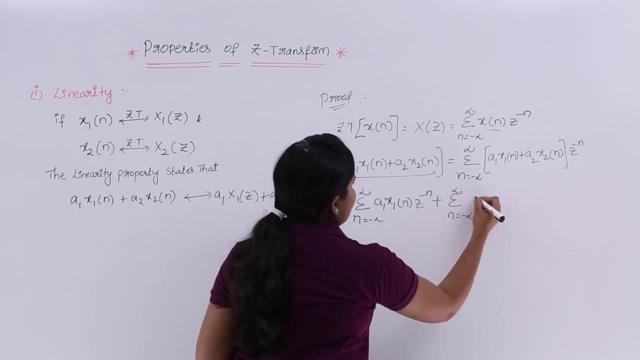 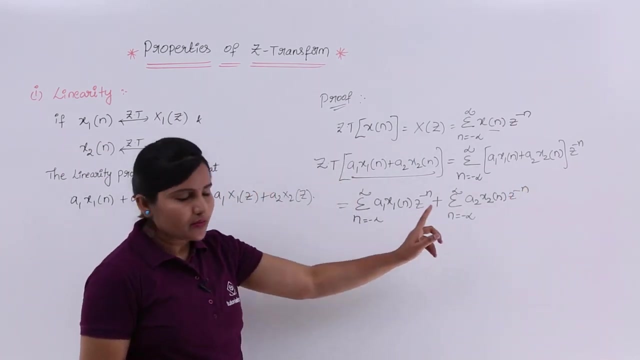 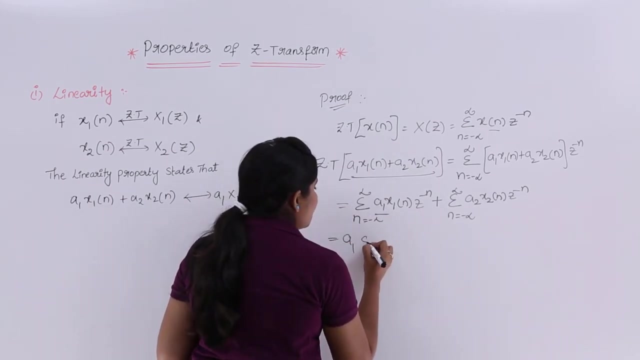 infinity to infinity. a1 x1 of n into z power minus n. This is one term. another term is summation n equivalent to minus infinity to infinity. So a2 x2 of n into z power minus n, This is another term. So now here a1 is a constant, So you can put it out. So a1 summation n is equivalent to: 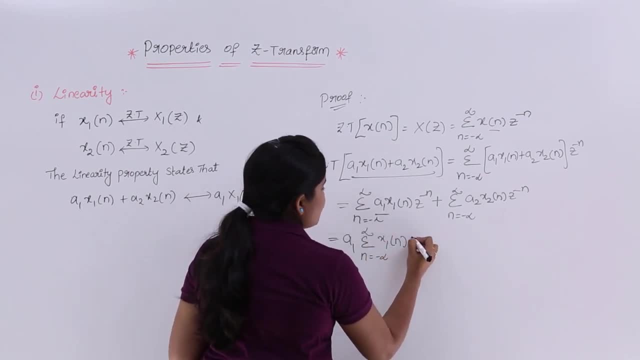 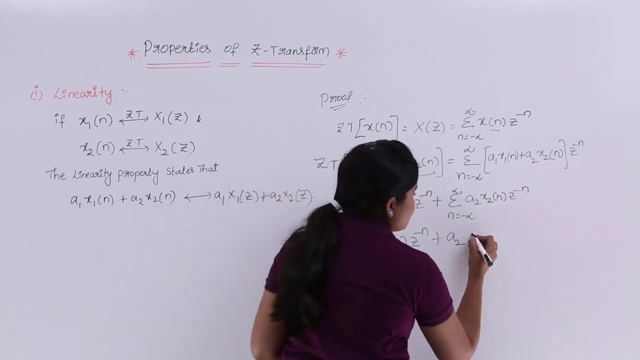 minus infinity to infinity. x1 of n z power minus n. this will be one term and here also a. 2 is also constant. I am taking it out. and summation n is equivalent to minus infinity, to infinity. x. 2 of n z power minus n. this is: